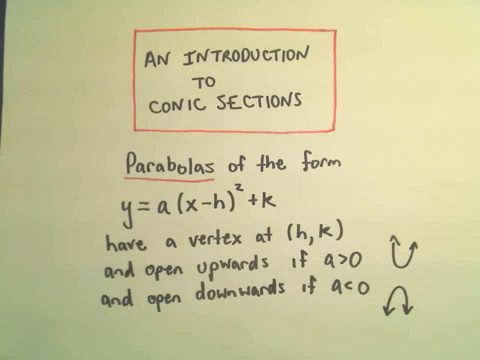 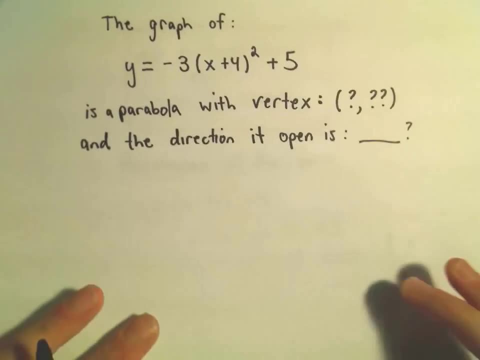 and it's going to open downwards if a is less than zero. So not both on the same graph, you just get one or the other. So a couple questions. So the graph of y equals negative 3 times x plus 4 squared plus 5,. 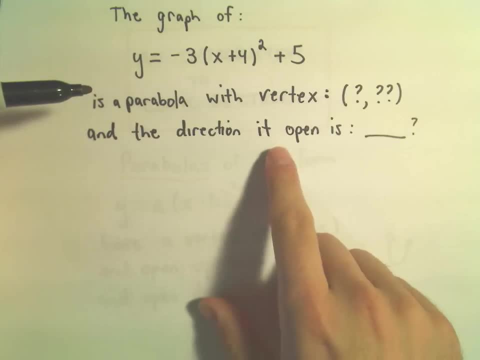 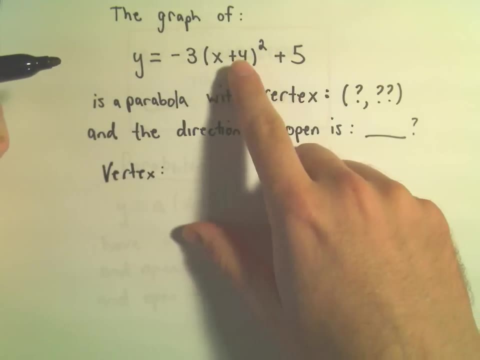 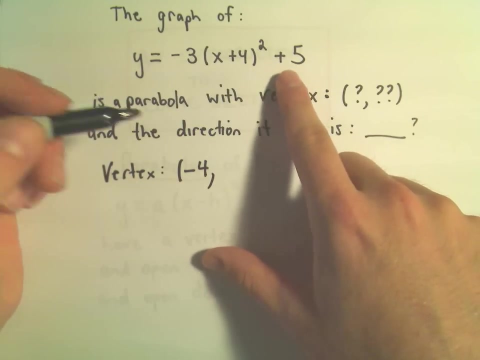 this is a parabola. with what vertex and in what direction does it open? Well, again, the vertex is not too bad when you have it in this form, Even though I see a plus 4, we use a negative, So the vertex is negative 4, but again, whatever the constant is that's being added or subtracted. 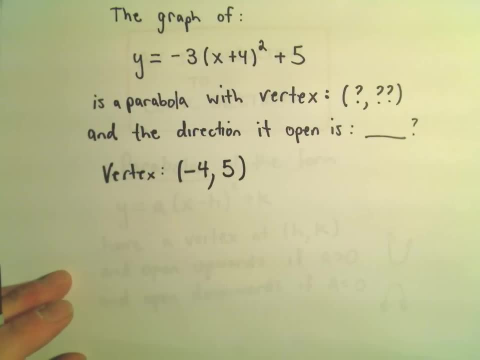 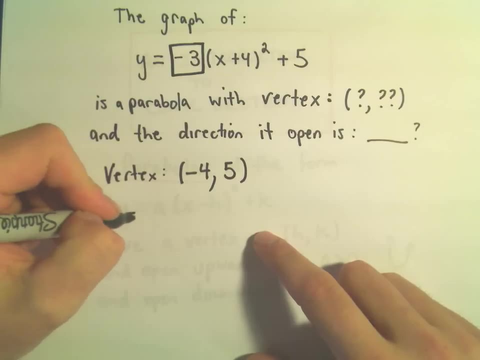 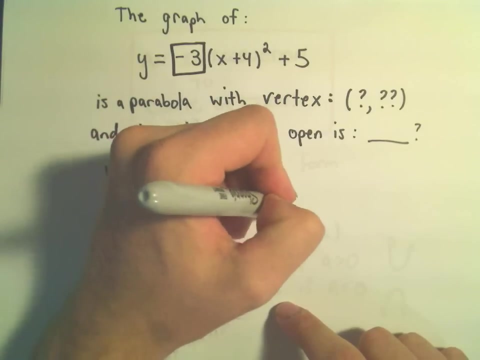 we actually use that one. So the vertex in this case would be negative 4 comma 5, and the a value is the number out front and in this case, since our a value is negative 3,, which is certainly less than zero, that's going to mean the parabola will open downwards. 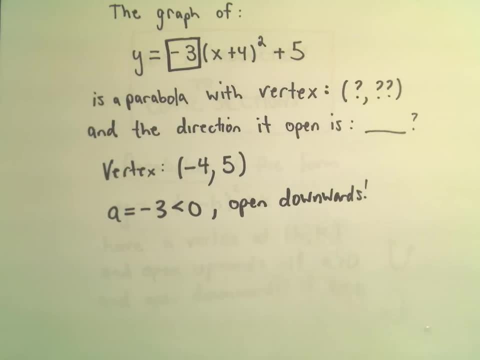 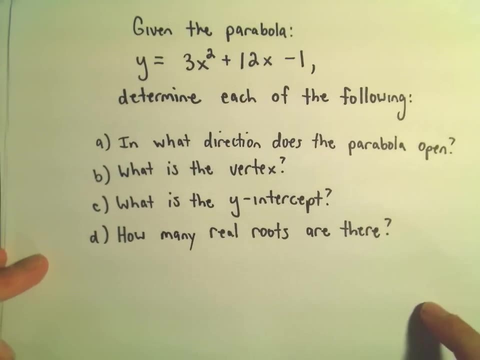 Okay, so no big deal, Just recognizing a formula. you know a type, a form, this form of a parabola. Another question here: so suppose we've got the parabola 3x squared plus 12x minus 1.. 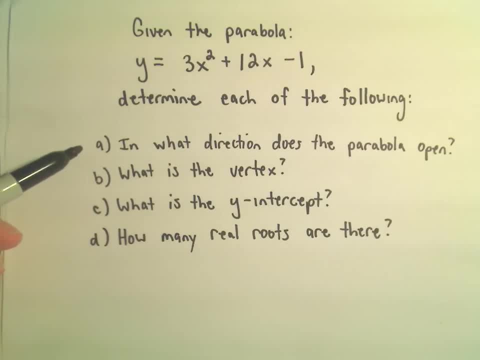 We want to know a couple things. In what direction does the parabola open? what's the vertex, what's the y-intercept and how many real roots are there? Well, in what direction does the parabola open? All you have to do is look at the coefficient on the x squared term. 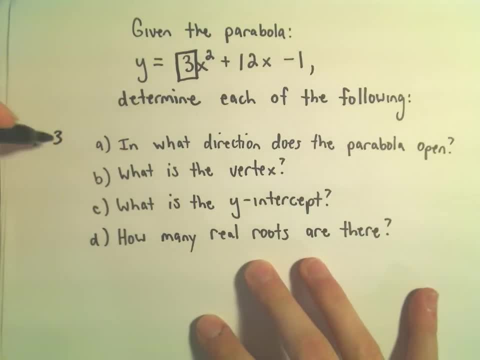 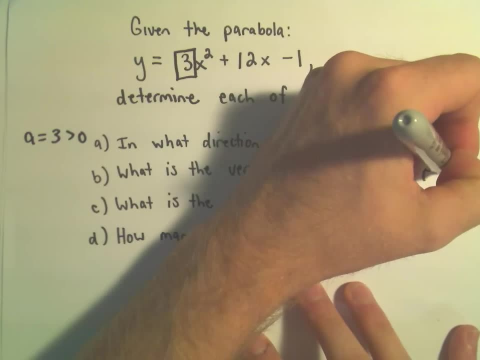 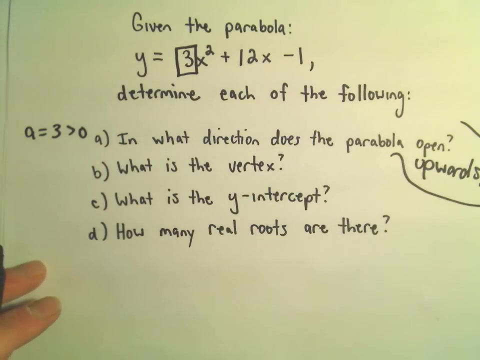 That's going to be your a value. So, in this case, since a is 3,, which is greater than zero, we would say that it opens upwards. Okay, so it opens upwards. We want to figure out the vertex. This is probably, to me, the hardest part of any of these questions. 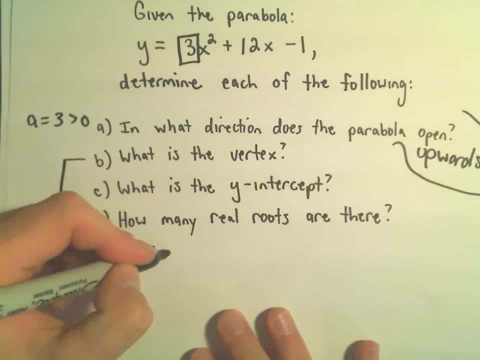 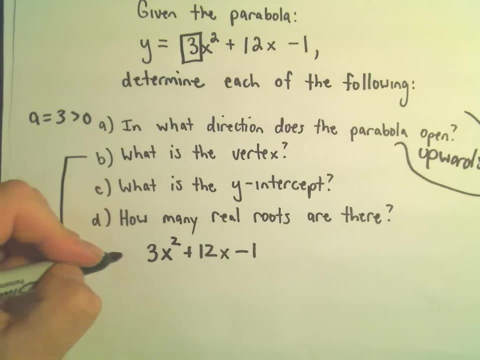 To figure out the vertex. what we're going to do is for this parabola, 3x squared plus 12x minus 1, what I'm going to do is I'm going to complete the square. Okay, on the right-hand side. 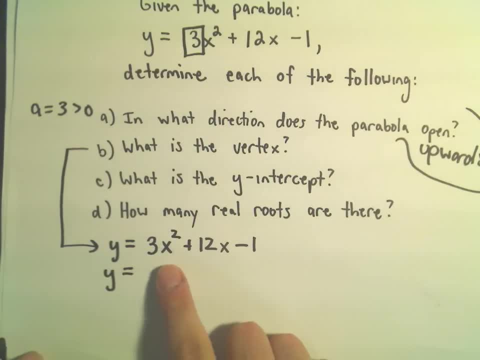 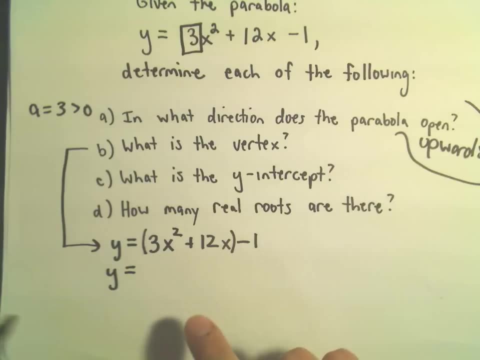 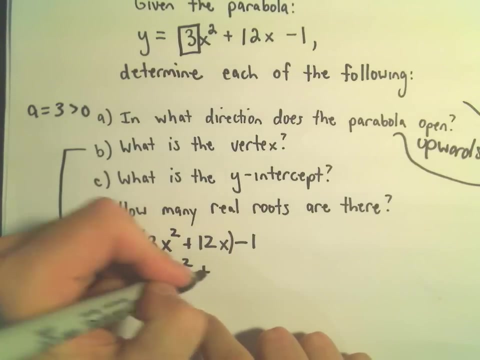 Okay. so the first thing I'm going to do is I group my x's together. I want the coefficient on the x squared term to be a positive 1, so, whatever the coefficient is, I factor it out. Well, 3 times x squared would be 3x squared, but then we would also have to change instead of 12x. 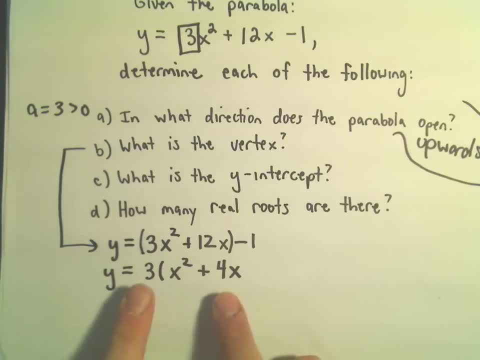 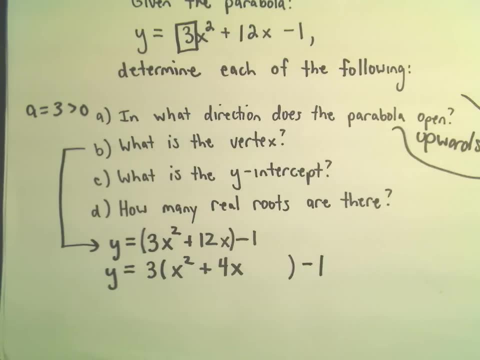 we would now have to make it 4x, So that gives me my positive 12x, But I'm going to leave myself a little room too, Okay, Because I'm going to do this completing the square step. Okay, a couple of things to be careful about. 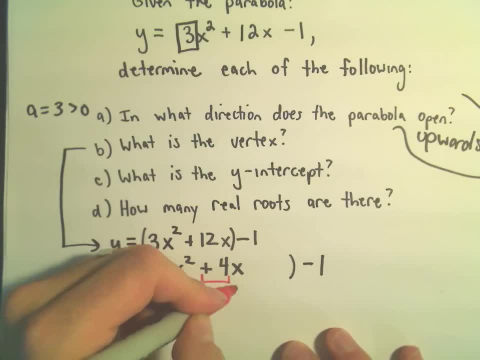 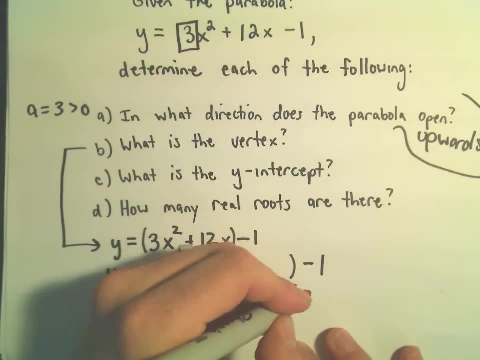 So the first thing we do is we take the coefficient in front of the x, which is positive 4.. That's going to give us a positive 2.. And then what we do is we take that number and we square it. That's going to give us a positive 4.. 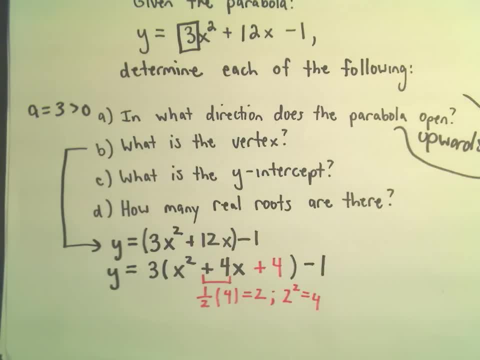 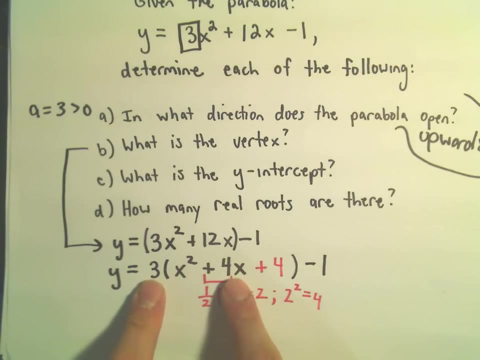 That's the number we put back inside the parentheses. So at this point we've changed our equation around. Okay, If you were to distribute everything out, we would get our 3x squared, which we had originally in the problem. We would get a plus 12x, which we originally had in the problem. 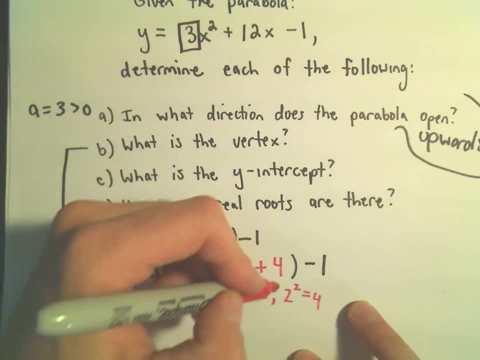 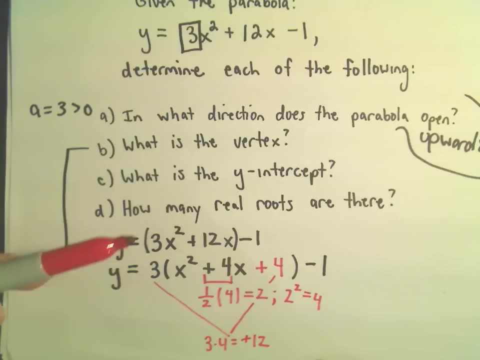 But notice, if we multiply our coefficient of a 3 and this value of a 4 we just got, we would end up getting a positive 12.. So really, what I've done is I've added 12 to this equation on the right-hand side, just kind of out of nowhere. 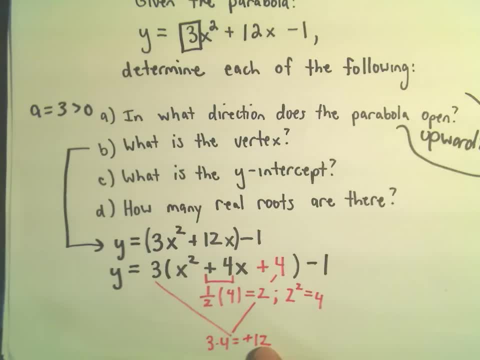 And that's okay. but we have to compensate for that And since we added 12, what we're going to do is we're going to subtract 12 from both sides. So again, you know, to me this is kind of the step that you know, a little less mechanical. 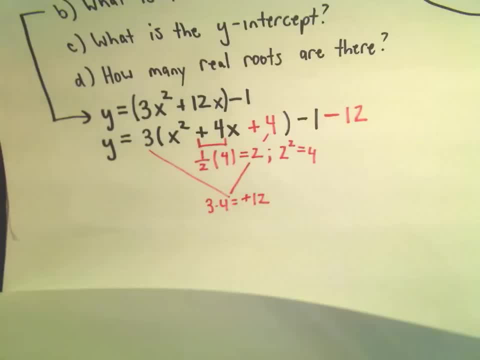 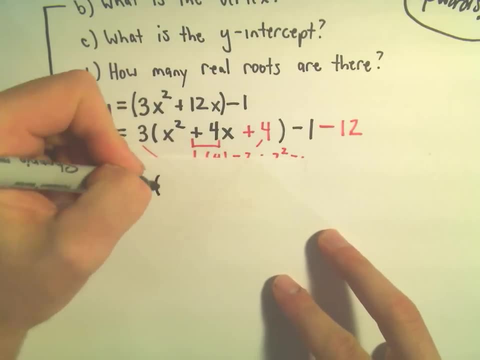 You really have to think what's going on here, just to make sure that you're getting all your coefficients and your values correctly. So at this point, though, the idea is we can factor x squared plus 4x plus 4 as x plus 2 times x plus 2.. 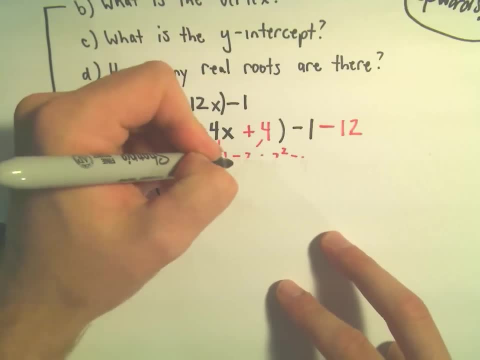 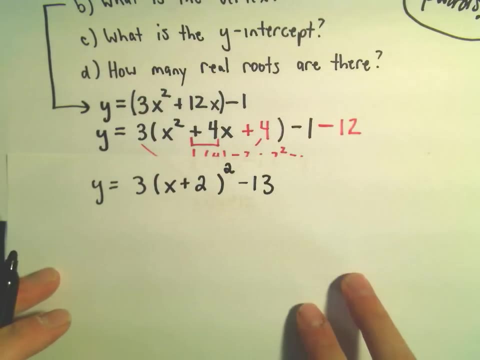 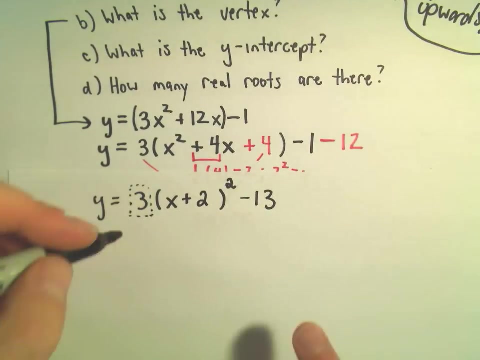 But we don't want to do that. Okay, So we can simply write that as x plus 2, quantity squared Negative, 1 minus 12 would be negative 13.. And now we have this in our vertex form. Okay, Notice, our a is the same a we picked out before. 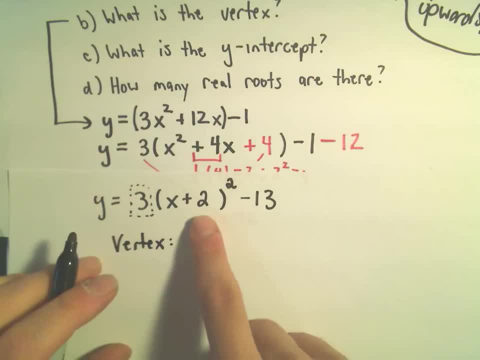 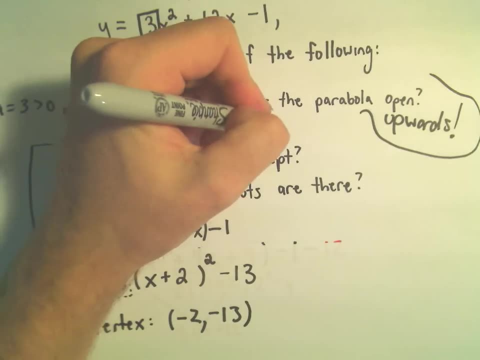 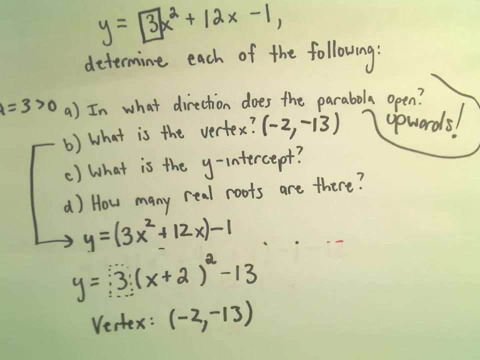 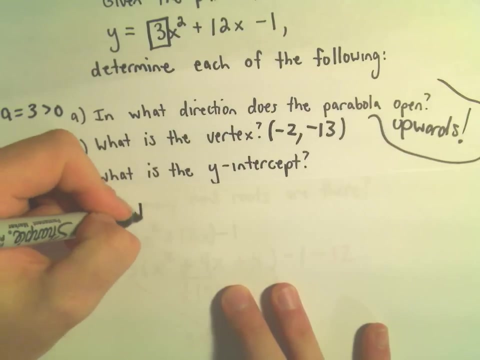 The vertex. in this case, the vertex would be negative 2 comma, negative 13.. So we've now figured out the vertex by writing it in this vertex form. Part C: what's the y intercept? Well, to get the y intercept, all we have to do. to get the y intercept, all we do is simply plug in: x equals 0.. 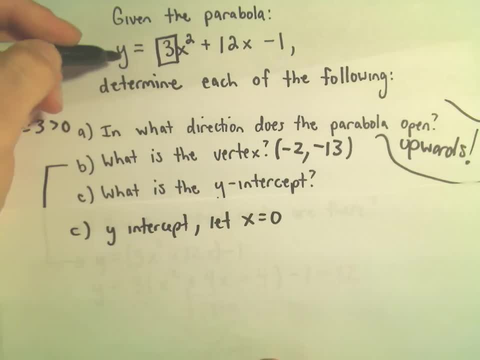 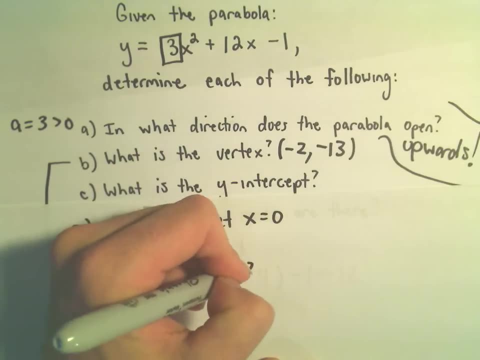 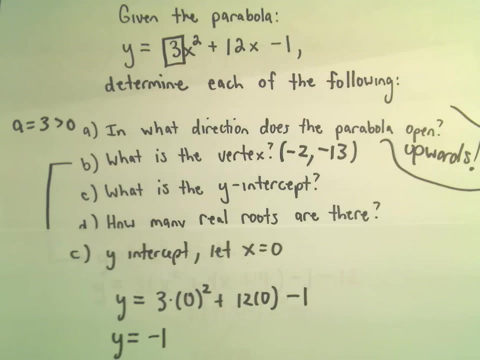 So if we plug in x equals 0 in our original equation, we'll get 3 times 0 squared, plus 12 times 0 minus 1.. Or we'll simply get a y value of negative 1.. So the y intercept is going to equal negative 1.. 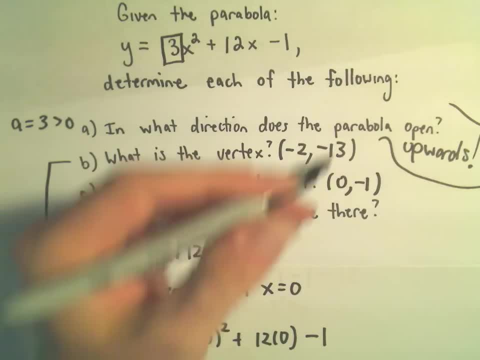 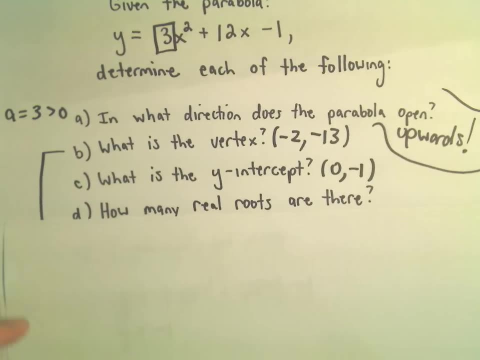 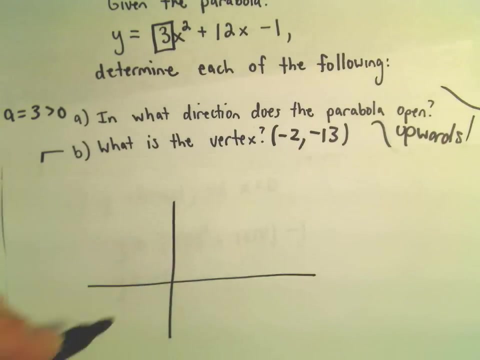 We could say it's at the point 0 comma negative 1.. And the last question here: how many real roots are there? So, without finding the real roots, I'm just going to make a geometric observation. We said the vertex was at negative 2 comma negative 13.. 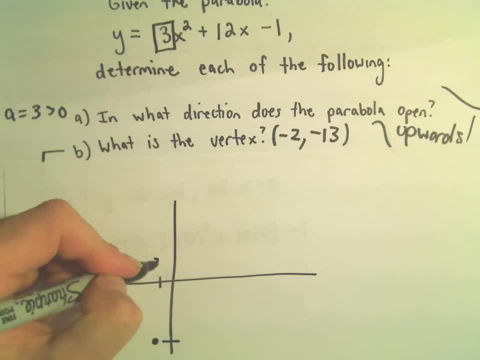 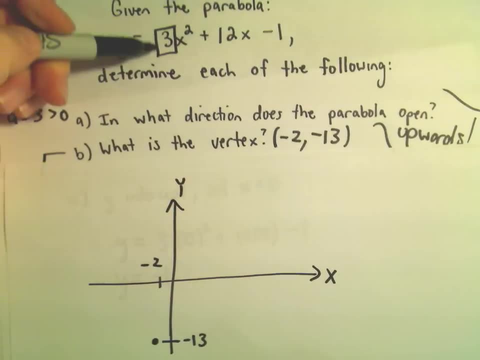 So negative 2 comma, negative 13,. I don't know, it's somewhere down there. But we also said that this parabola, because of the coefficient on the x squared term being positive, we said, since it's positive, it's going to open upwards. 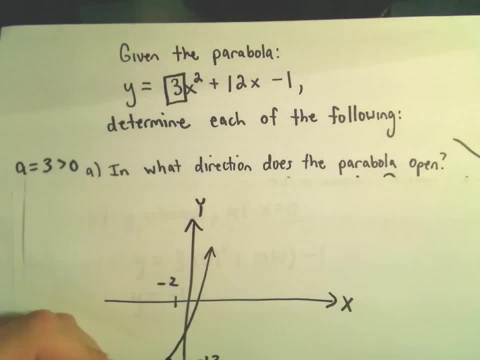 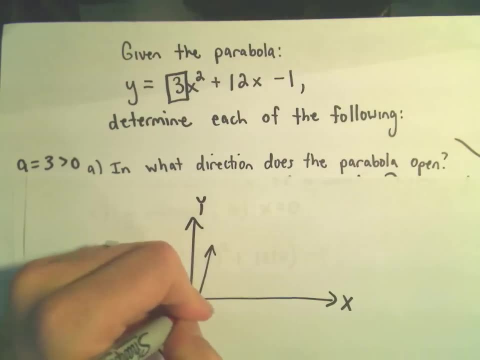 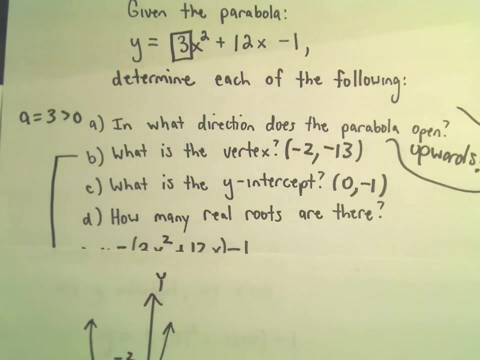 And since it opens upwards, well, that means in this case it's going to have to cross the x axis at two places. And since it crosses the x axis at two places, I would say, well, since that happens, there has to be two real roots. 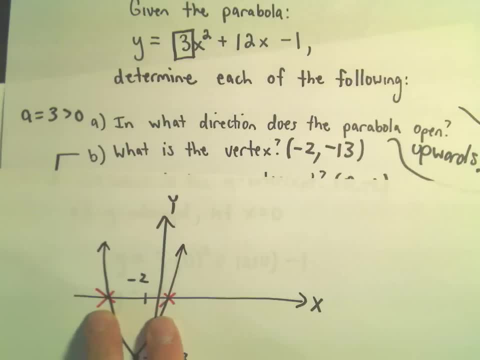 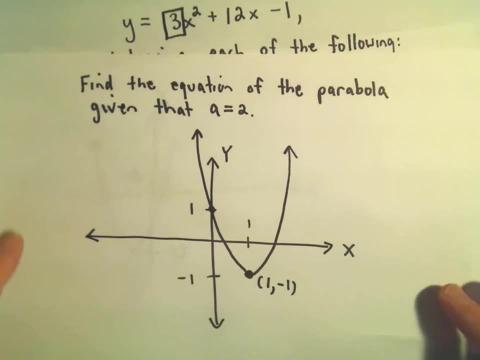 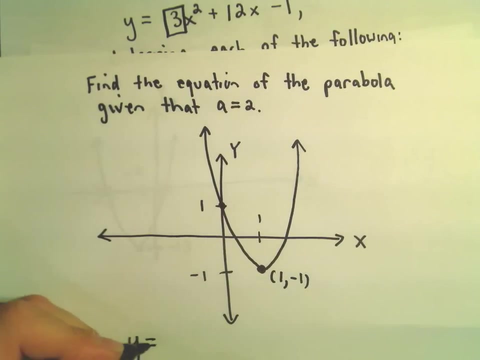 Okay, Crosses the x axis twice. that means there are two real roots. One more quick problem here. Suppose we want to find the equation of this parabola, given that we know that a equals 2.. Well, all we have to do. we know our formula for a parabola is a times x minus h, quantity squared plus k. 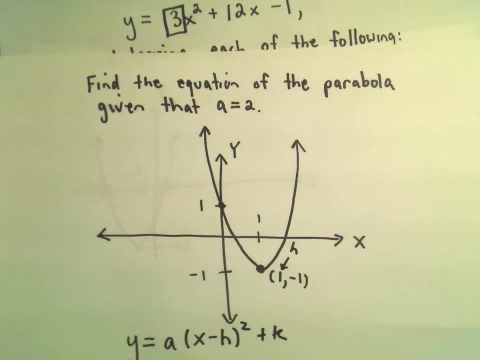 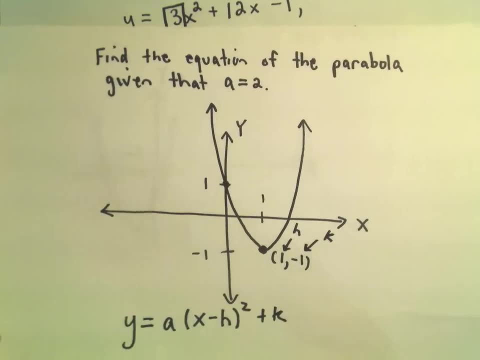 Well, in this case, my h value is positive 1, because that's the x coordinate of the parabola, My k value is negative 1, because that's the y value of the vertex, And at that point we're given everything we need.